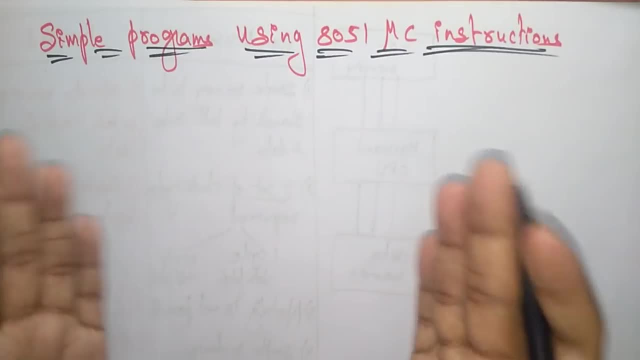 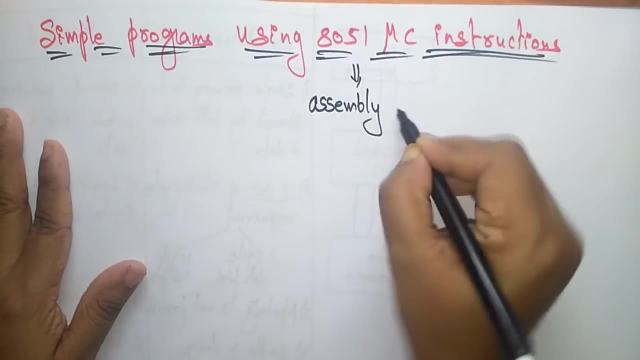 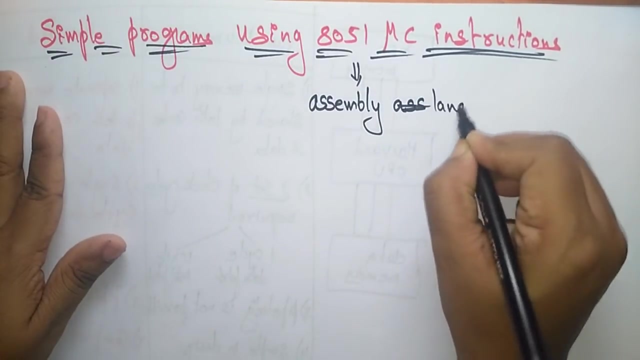 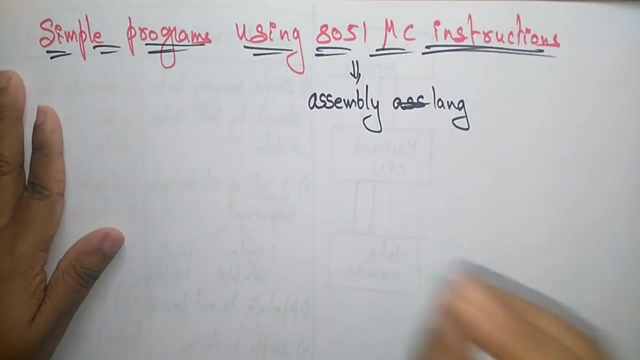 So 8051 microcontroller means we will use the assembly language. The programming language that we used for 8051 to programming 8051 is the assembly language. So this assembly language is fully hardware related programming language. Assembly language is a fully hardware related programming language, Remember. So, whatever the file you are taking, 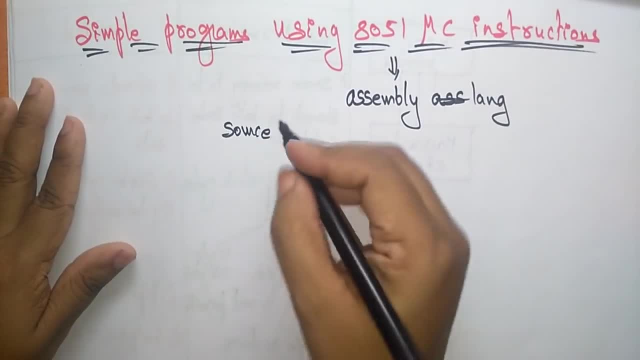 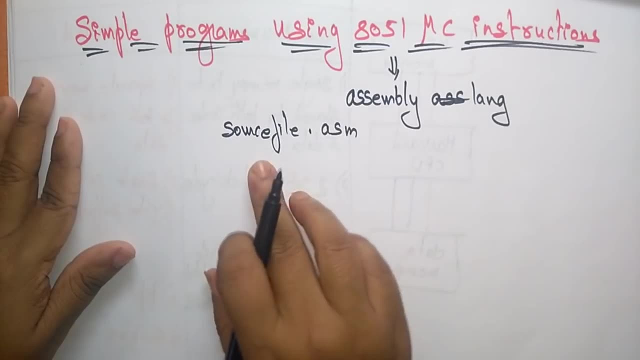 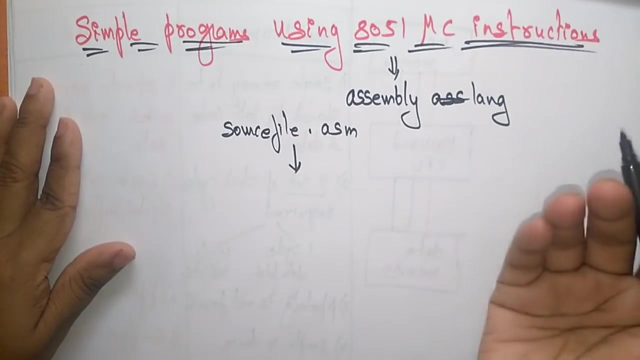 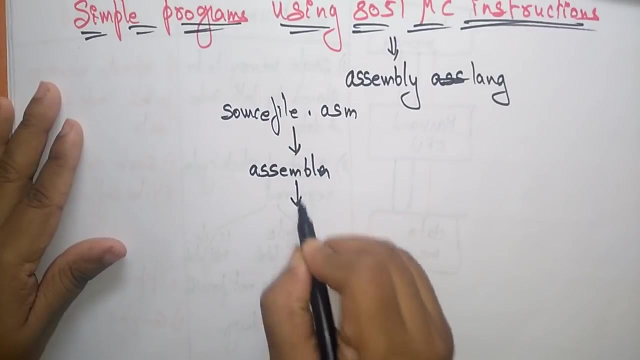 so that file has to be stored, as suppose. let's take source file. Source file dot ASM. The extension is assembly language, ASM. Save the file as dot ASM. Source file: dot ASM. So after that, after saving the program, you need to assemble it. It is by the help of assembler And next linker, And finally you will get the executable file. 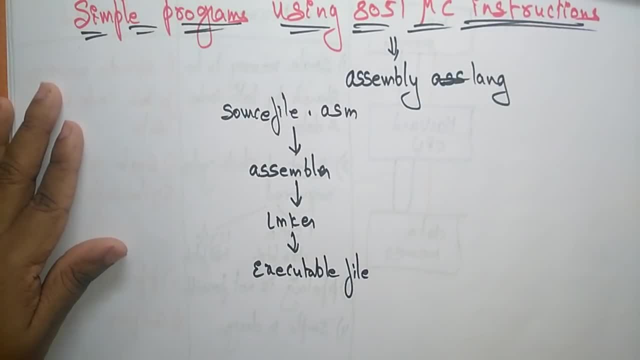 So this is a process, how the program is going to be executed. So you are writing the source file in the form of assembly language That is in the mnemonics. with the help of the mnemonics, And the assembler is going to convert this assembly language into OBJ file. 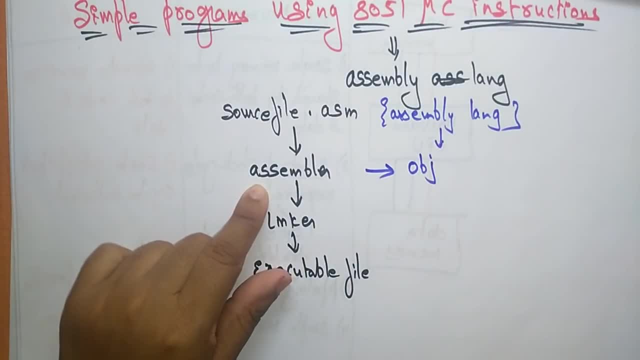 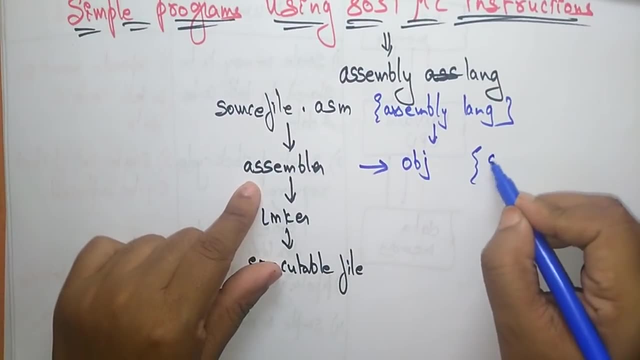 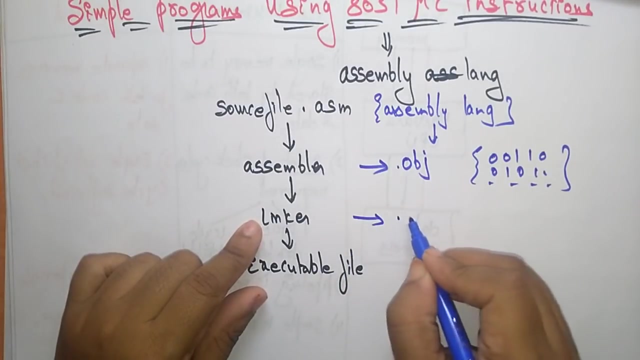 Okay, So the assembler is nothing but the conversion of dot ASM file into dot OBJ file. Source file: dot OBJ. So OBJ means is in the form of machine language language. Yeah, Yes, Yeah. 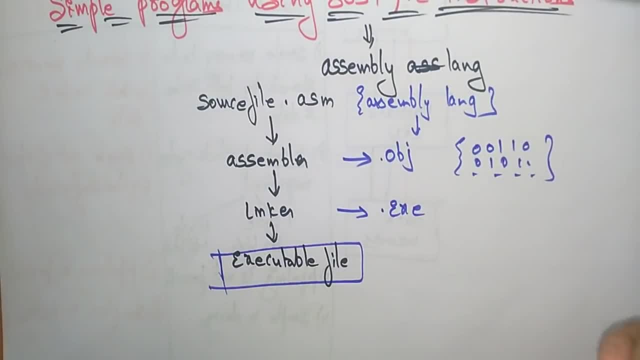 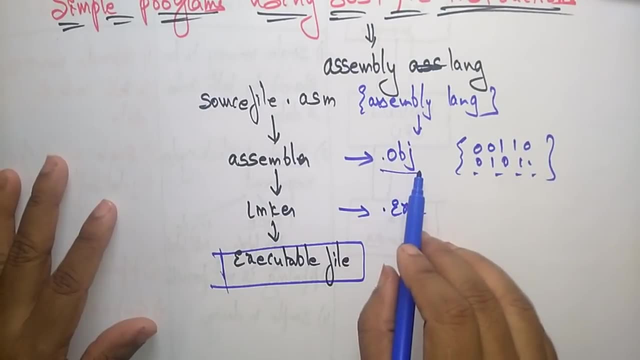 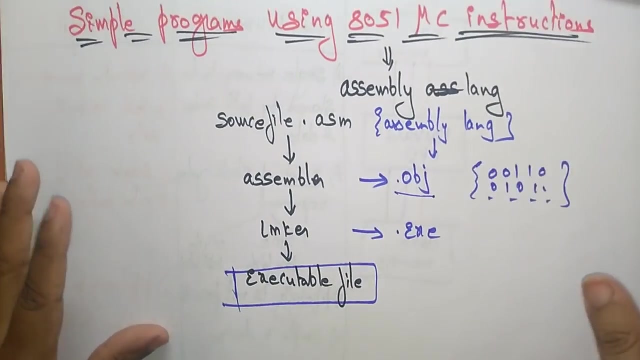 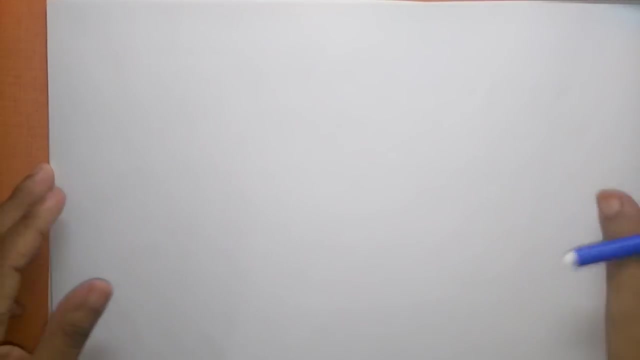 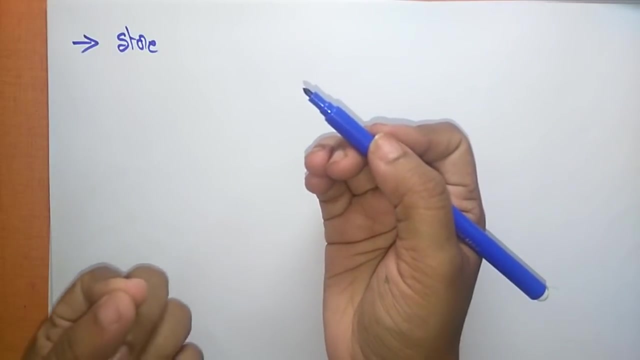 obj file. after that it links. the program means the executable file, dot, exe file. so let me explain the simple programs by using the instructions, the instructions that are present in the 8051 microcontroller. the first one: what you will, what type of assembly code you will use to store. 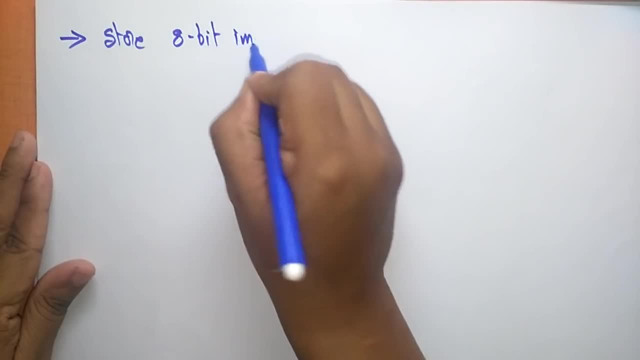 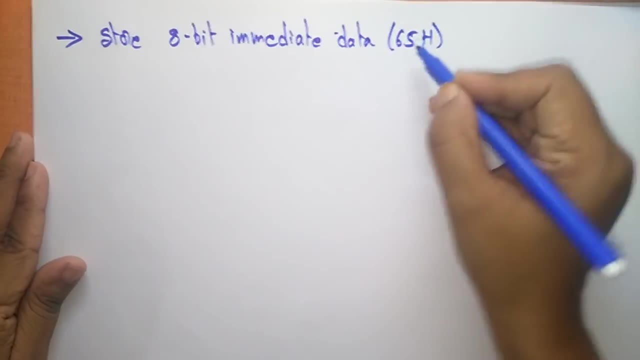 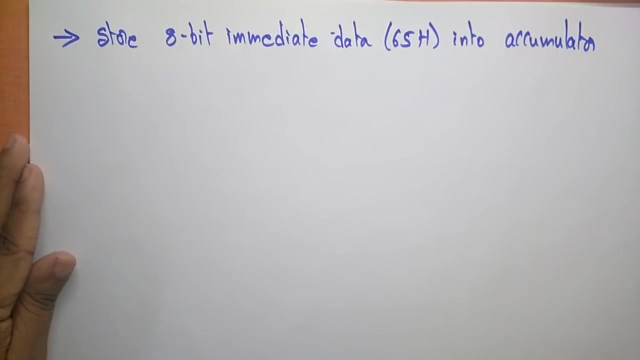 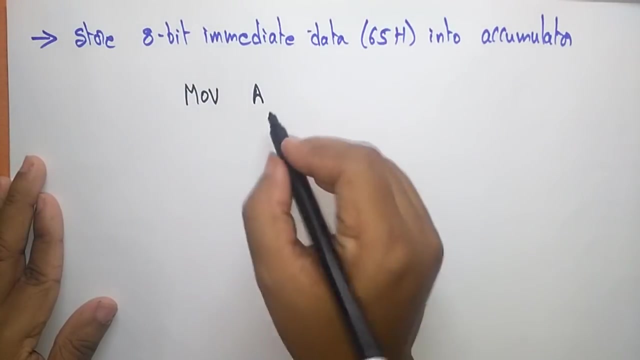 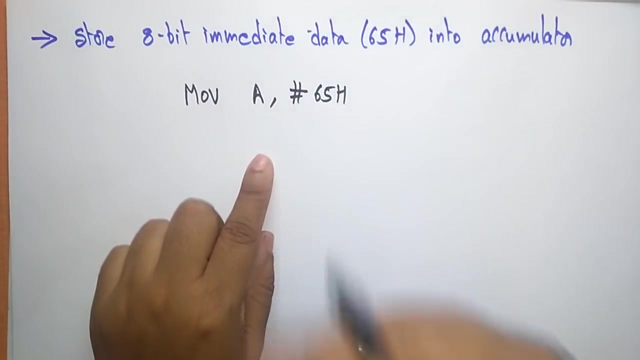 8-bit immediate data. let's take 65 H into accumulator. so I want to store the 8-bit, that is a 65 heat H, into accumulator. so what is the? the mnemonic code you have to write: move 8 a is a accumulator, a comma: hash 65 H. hash 65 means immediate data, whether it is an address. 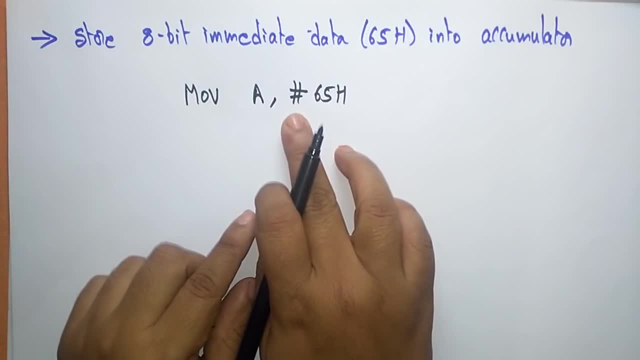 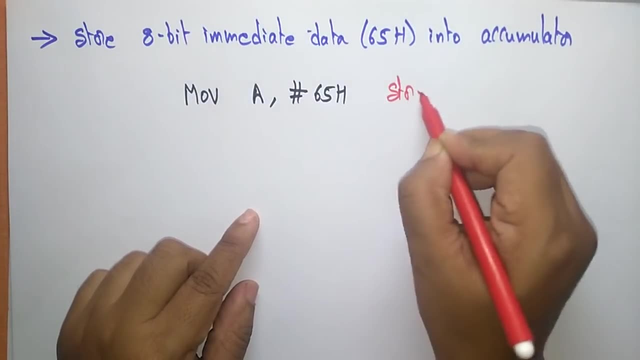 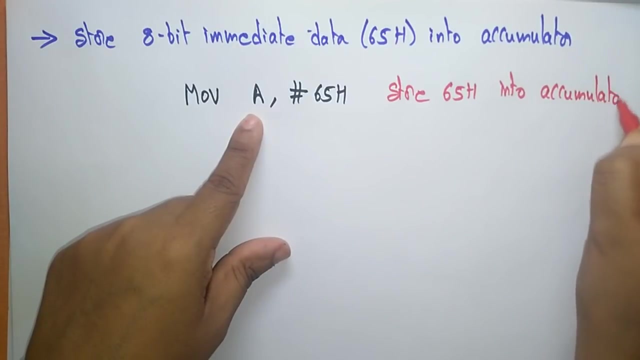 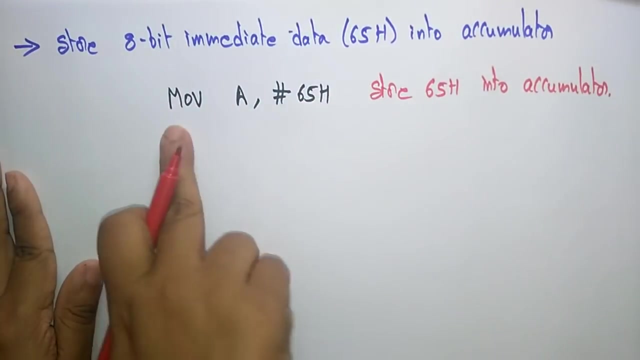 or data hash. that is a immediate. so to represent the immediate data you have to represent it as a hash. so what it is doing, it stores, store 65 H into accumulator, accumulator. a means accumulator, so 65 data is stored in a. so for the, for this statement, you have to write the code as move, a comma 65 H. so let's take 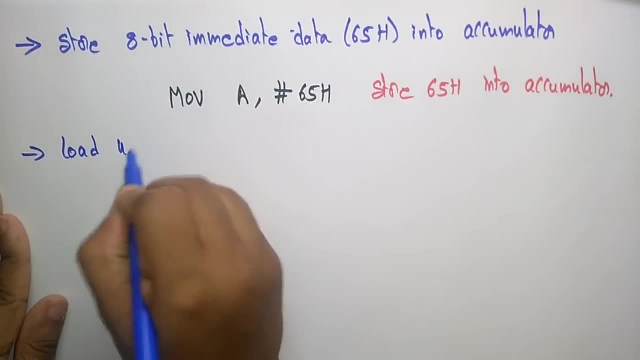 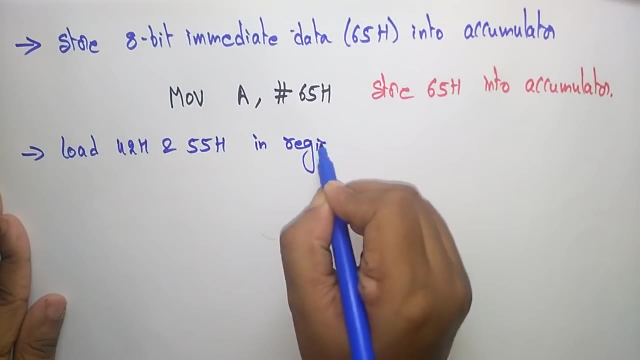 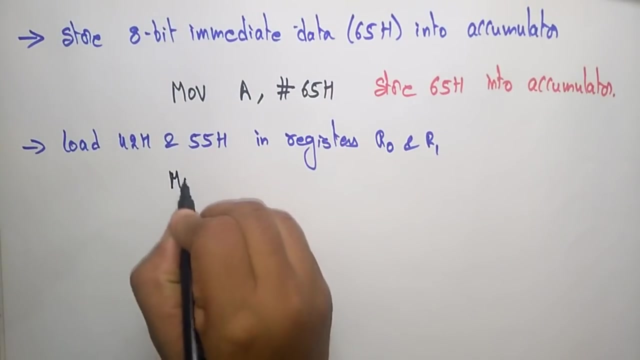 if you want to load load 42 H and 55 H, let us take in registers R, naught and R1 respectively. so how you load the values of 42 and 55 in R, naught and R1 registers. so for that you need to write the syntax move. 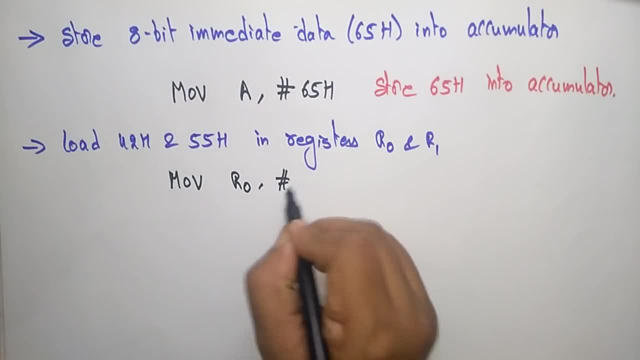 R naught comma immediate data. that is the 42 H move R1 comma hash, 55 H. so from right side to left side. so the data that is present on right side is moving to the left side. so here it represent it, going to load 42 H in R knots register and load 55 H and 55 H as시에ge. coming to the left side. so here it represents it, going to load 42 H in R naught register and load 55 H for 22H movies a day. 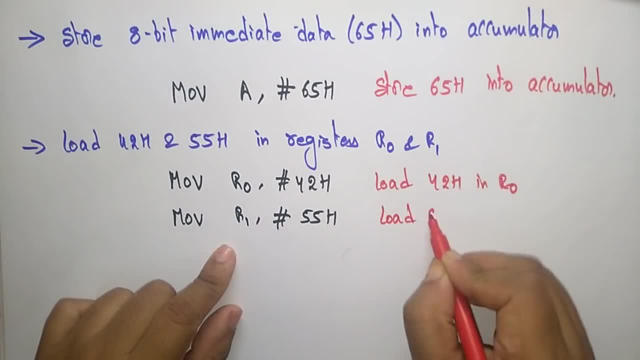 you need to enter 기 ahh. so subsequent code to prayer H acc is darip kha E move r1 comma hash percent, so pm to meaningless. so if you are correct, if you want to do this, let us tell that problem. rejammin chaos again in a software the already has been solved for this. 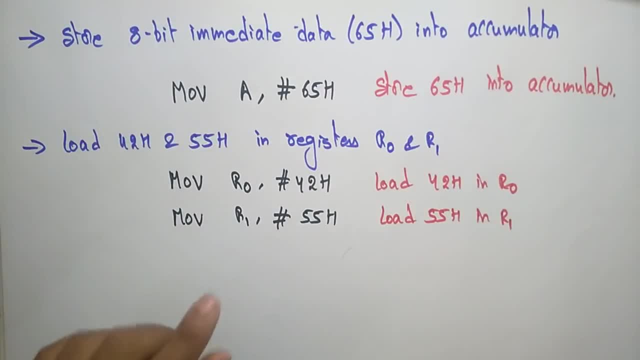 project управ, Yet keep it inside beads value fixed. so r1 h has 50 H. oh, certainly the elective code. so let us take a few more 55 H in R1 register. So here I am just explaining how we are going to use the instructions, the registers for writing the programs. 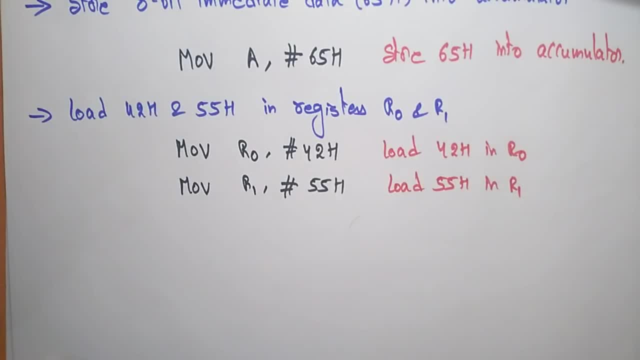 And the next program. let me take Now. I want to place the content of external memory location into accumulator. So whatever the external memory location is there, that location has to be placed in accumulator. So far, we have just moved the data, not the address. 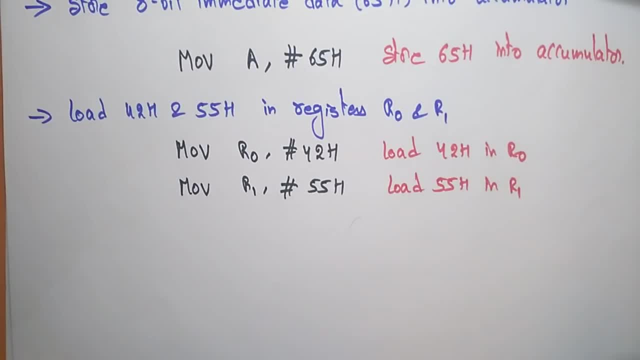 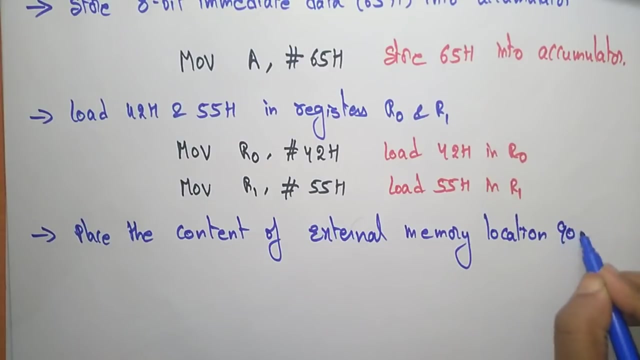 So now I want to place the external memory location into one of the register Place, the content of external memory. So in the external memory some data was there that has to be moved to accumulator. So here, external memory location, let us take 9000 H into accumulator. 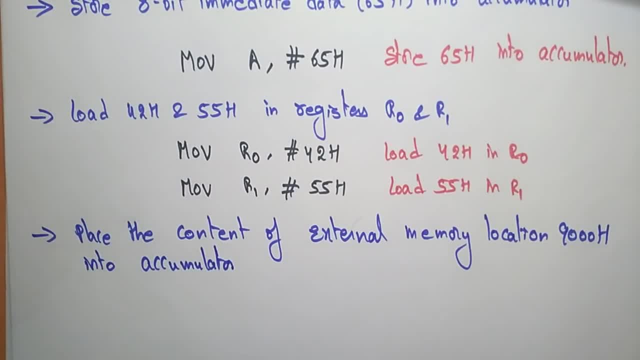 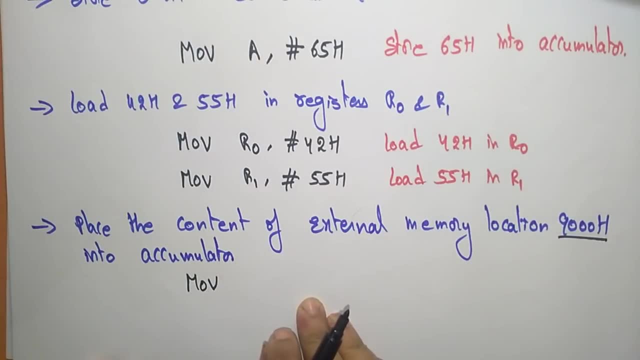 Accumulator means. So for this you need to write: So first move. whatever the external memory location is there that has to be moved into the data pointer DPTR, comma hash 9000 H. After that you need to write: move X A comma at the rate of DPTR. 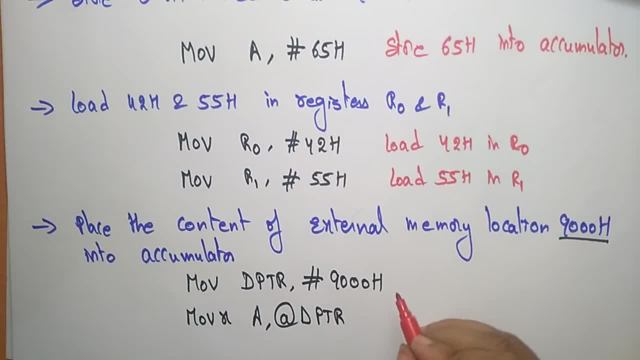 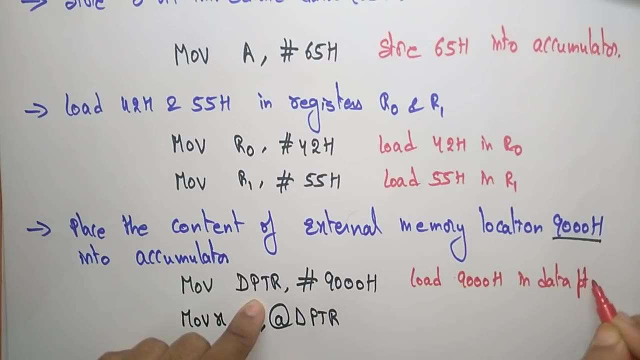 So what it means Here it just loads. So the load 9000 H in data pointer. So DPTR is a data pointer, Load 9000 H in data pointer register. That is immediate. So now the data pointer contains the 9000 memory location. 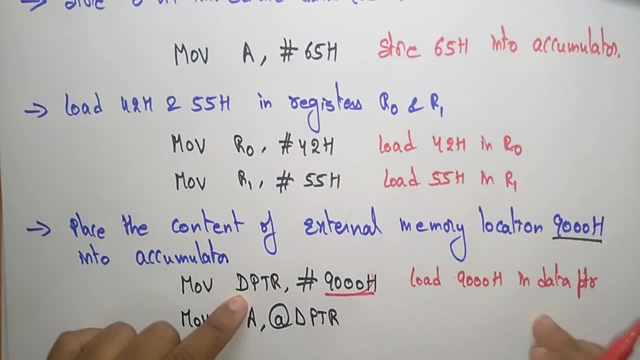 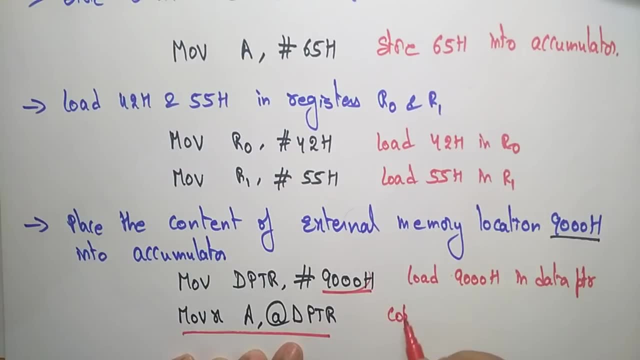 9000 memory location is stored in the data pointer. Load 9000 H in data pointer immediately. So what this syntax means. So here copying the at the rate of DPTR means in this location some data will be there. 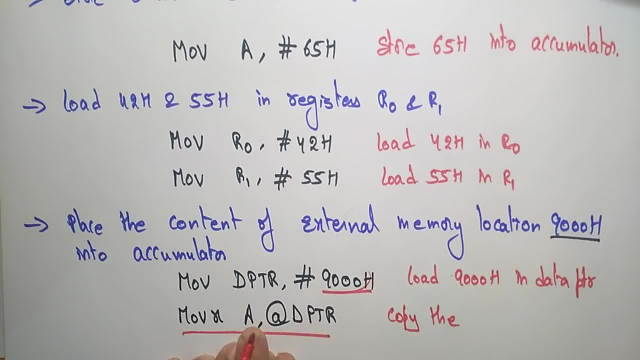 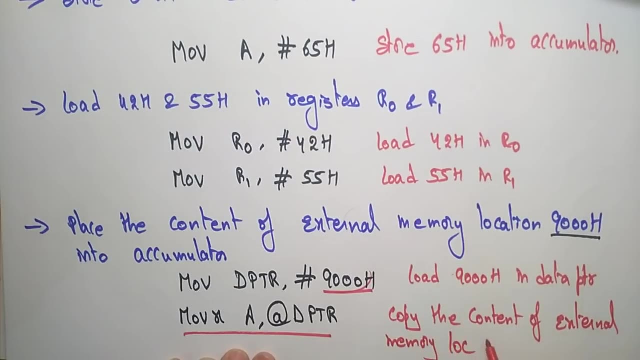 It means that 9000 location some data is there, That data has to be moved to the accumulator. Copy the content of content means data, The content of external memory location 9000 H into accumulator. So whatever the data that that is present on this 9000 location, that data has to be moved to accumulator.